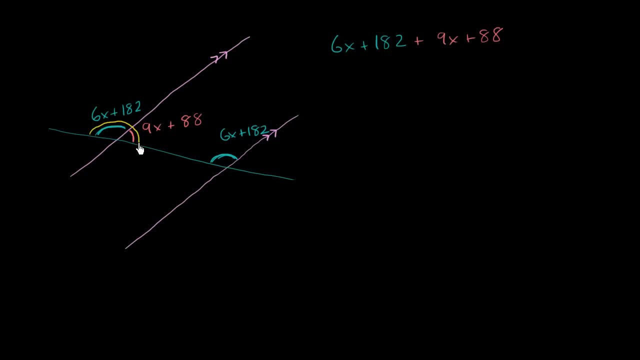 is going to be equal to 180 degrees. Now we just have to simplify this thing. So 6x plus 9x is going to give us 15x, And then we have 182 plus 88.. Let's see, 182 plus 8 would get us to 190. 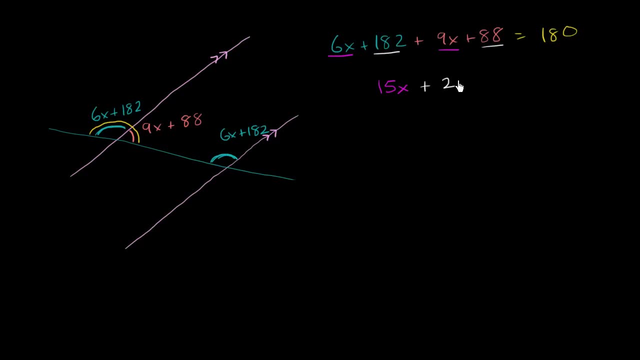 And then we add another 80, gets us to 270.. Plus 270 is equal to 180.. If we subtract 270 from both sides, we get 15x is equal to negative 90. And now we can divide both sides by 15.. 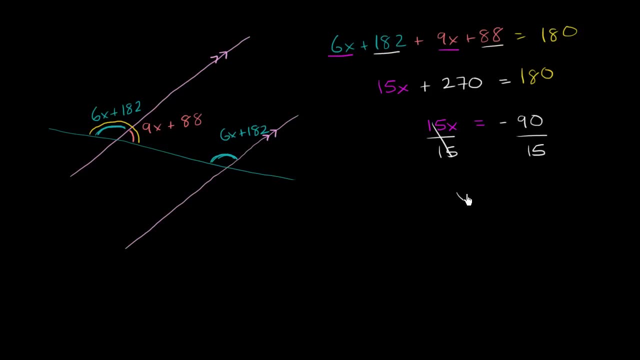 And we get x is equal to what is this? Let's see: 6 times 15 is 60 plus 30 is 90. So x is going to be equal to negative 6. So so far we've made a lot of progress. 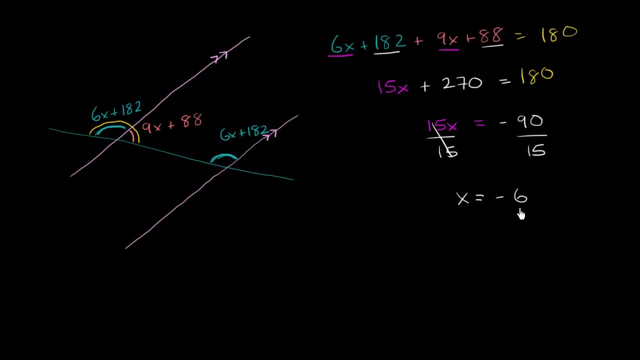 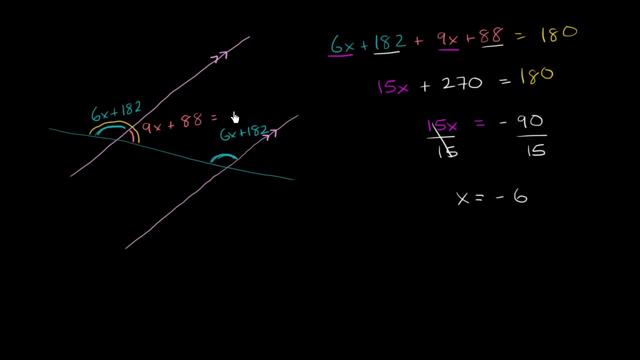 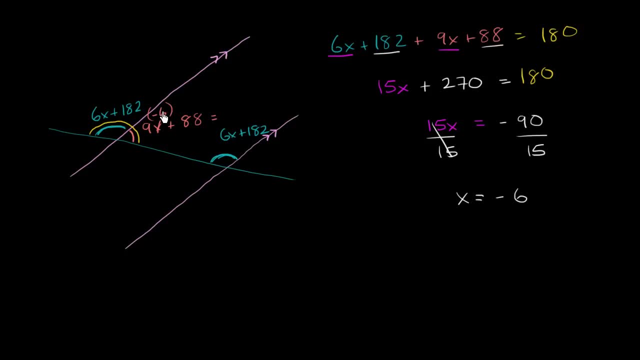 9 times negative. 6 is negative 54. Negative 54 plus 88. Let me write this down before I make a mistake: Negative 54 plus 88 is going to be. let's see, to go from 88 minus 54 will give us 34 degrees. 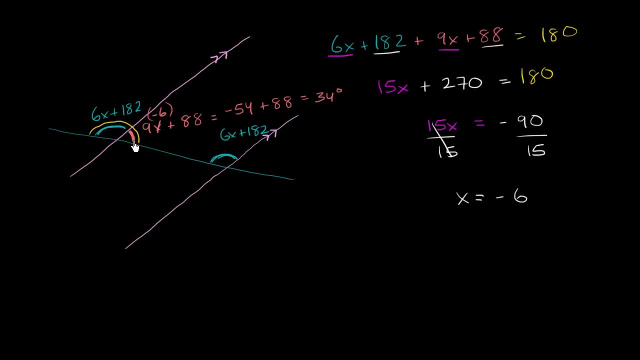 So this is equal to 34.. And it's in degrees. So this orange angle right over here is 34 degrees. The blue angle is going to be 180 minus that, But we can verify that by actually evaluating 6x plus 182.. 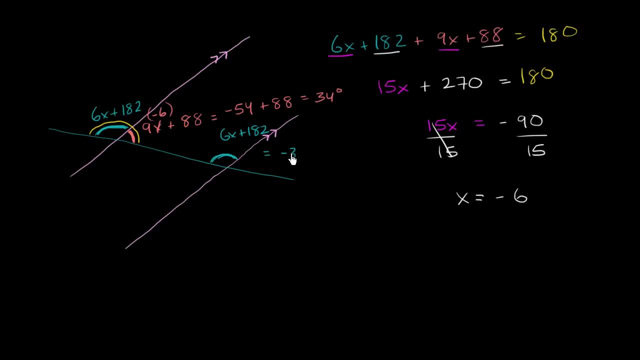 So this is going to be equal to 6 times negative. 6 is negative 36 plus 182.. So this is going to be equal to: let's see it's 1.. Let's see, if I subtract the 6 first, I get to 176..